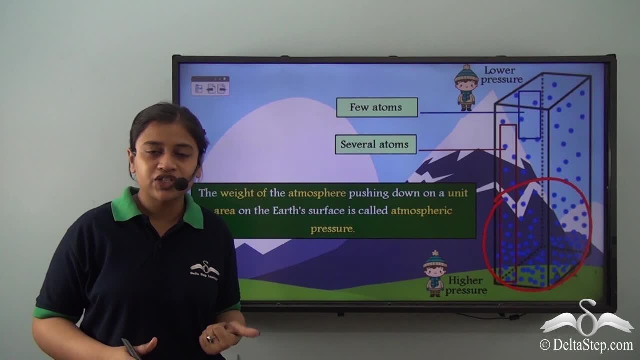 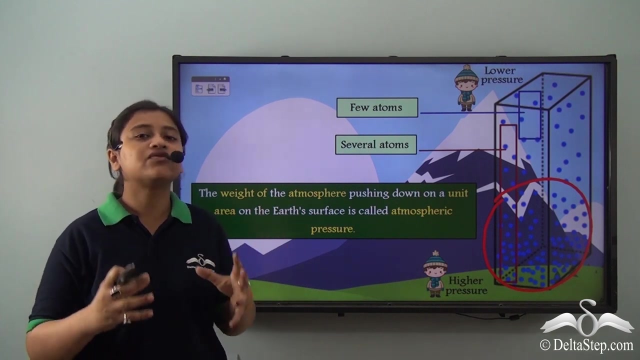 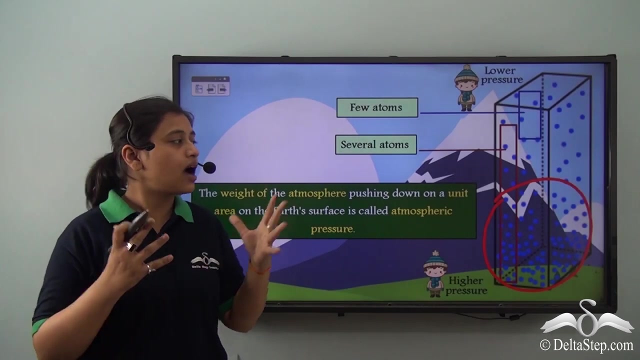 that influence weather. We have learnt how temperature, cloud cover, precipitation and humidity affects or influences weather. Similarly, there's another very important factor that influences weather, and that is the atmospheric pressure. So far, we have been talking about the concentration of air molecules in the lower layers and that the amount of oxygen 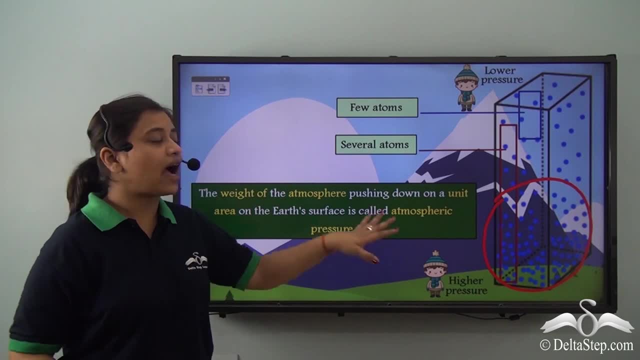 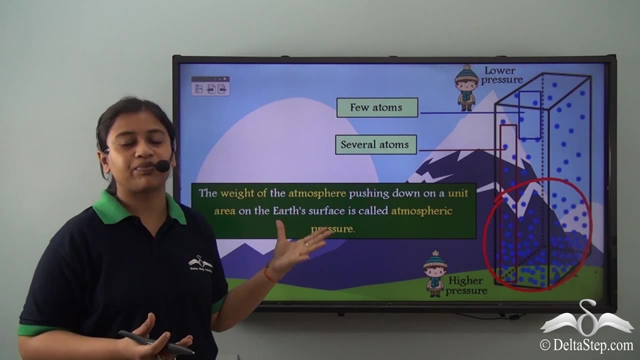 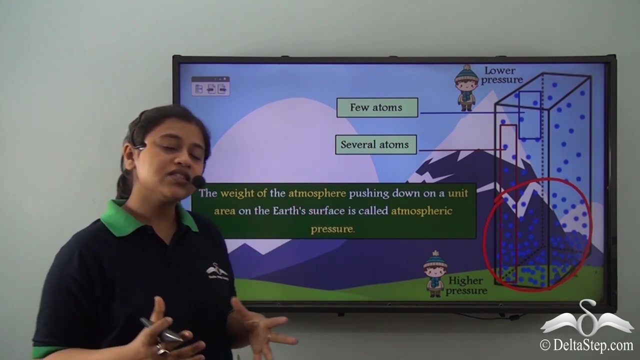 is more on the lower layers than on higher altitudes, But then why are we talking about this when we are going to talk about atmospheric pressure? It is all connected. So what exactly is the atmospheric pressure Now? since the concentration of air molecules is more on the lower layers, the amount of 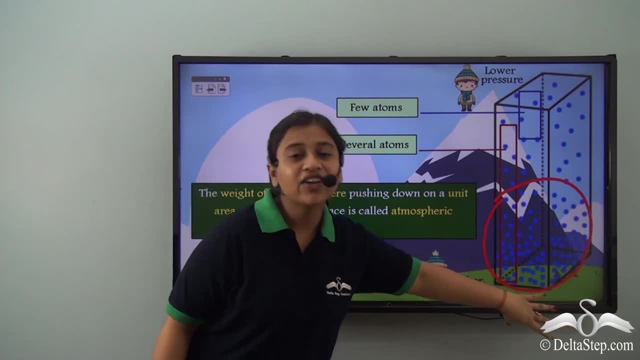 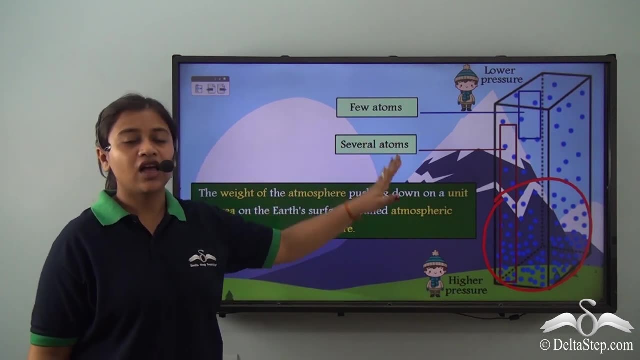 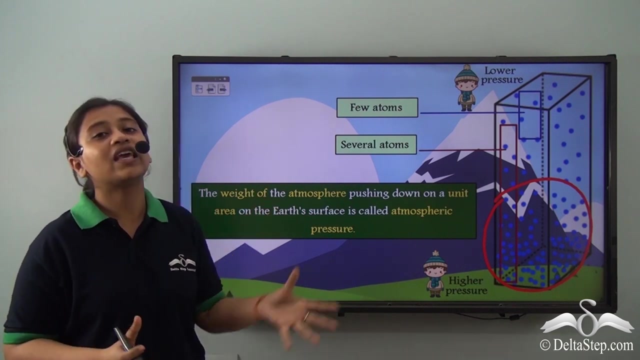 weight that it puts on an unit area of the earth's surface is more on the lower altitudes than on the higher altitudes. So, for example, you are on land, So the atmospheric pressure is nothing but the weight of the air on that unit area of the earth's surface where you are standing. So the place you are standing, you experience certain amount of atmospheric pressure. However, as you go up higher in mountains or hills, the amount of weight of that air on you tends to decrease, So the pressure on you is much less on higher altitudes. 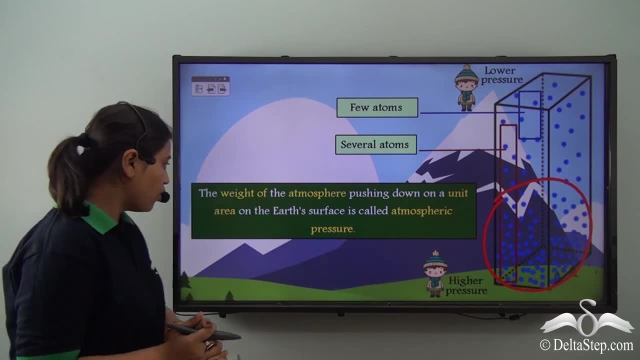 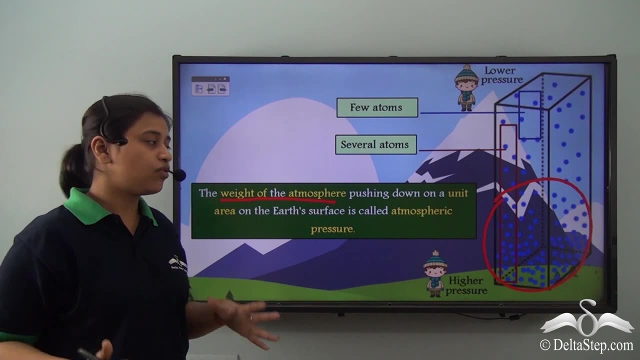 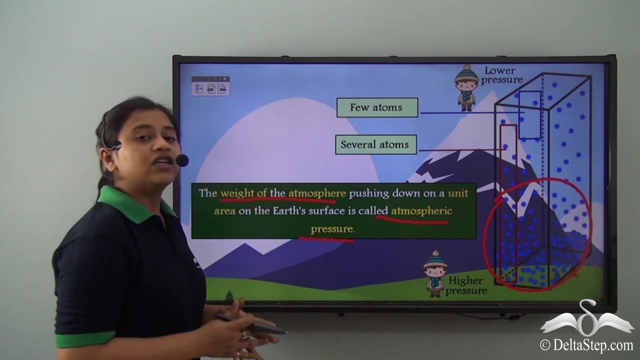 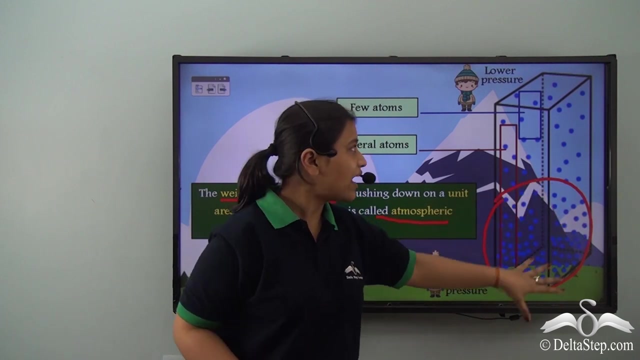 than on lower regions. So to define atmospheric pressure we could say that the, the weight of the atmosphere pushing down on a unit area of the earth's surface, is called the atmospheric pressure. This only means that the weight of the molecules on the lower regions is much more than on higher altitudes. So the pressure or the atmospheric 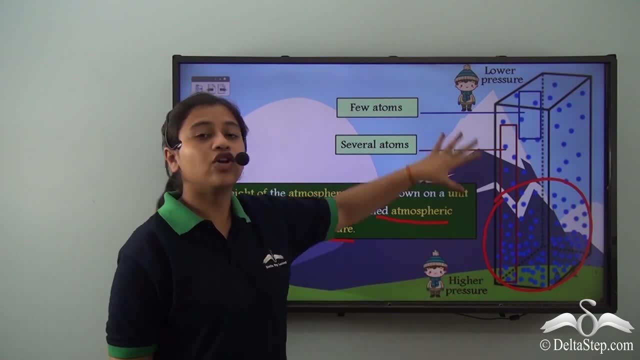 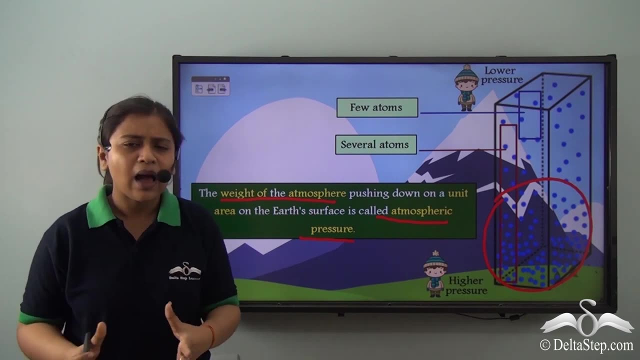 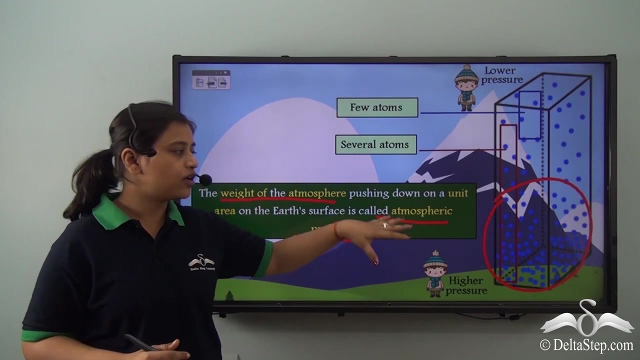 pressure is higher here, while it is lower on high altitudes. So this is how atmospheric pressure works. But now, how is this connected to weather? So, because of the difference in the atmospheric pressure in lower regions and in higher altitudes, people who have breathing- 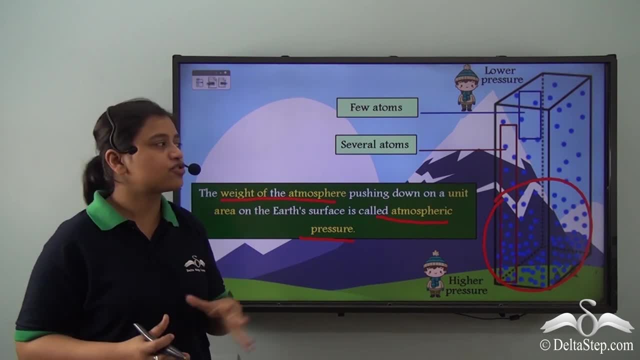 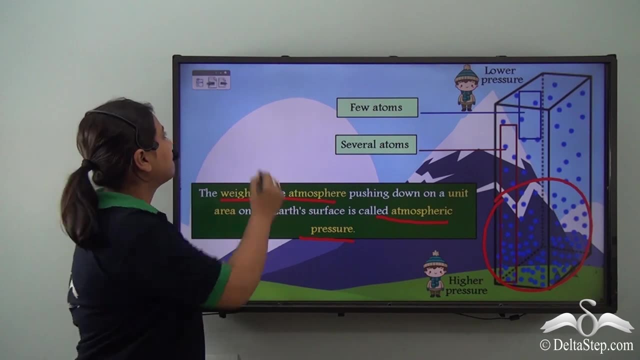 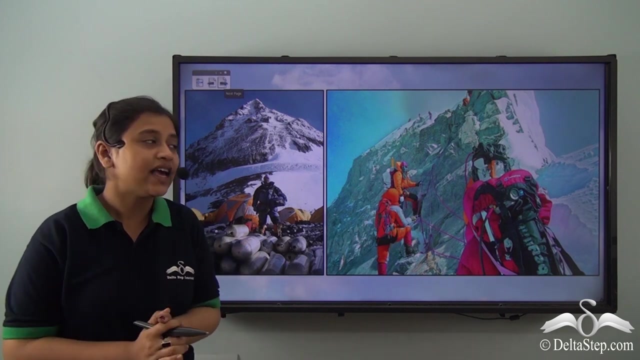 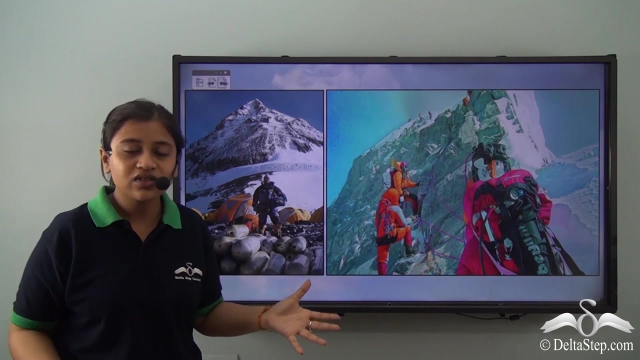 issues, or people who are old tend to avoid trips to higher altitudes or take a lot of precautions while planning a trip to such high altitudes. So here is another example where you see that mountaineers or people who love to hike in such snowy, icy mountains tend to carry huge cylinders of oxygen, As we just understood. 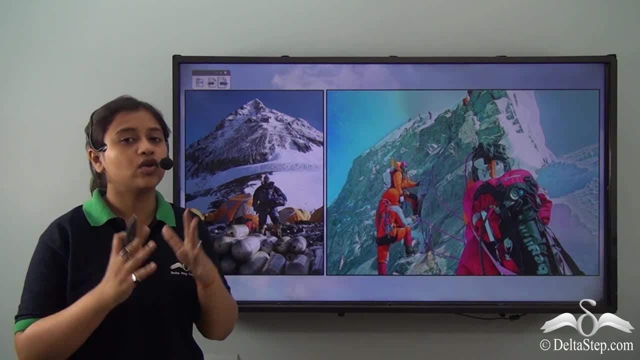 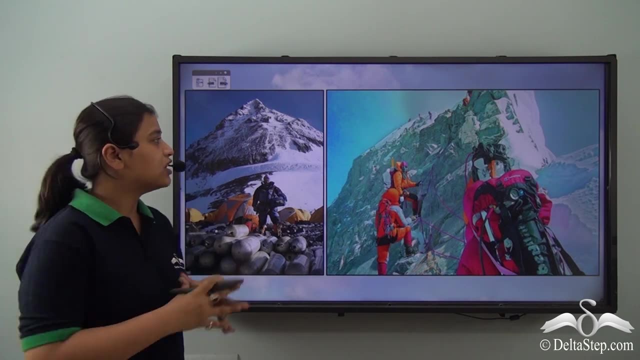 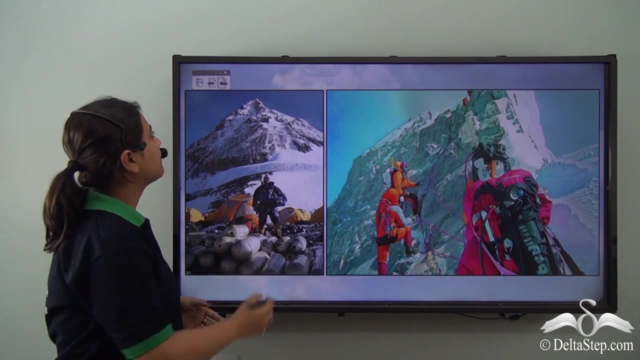 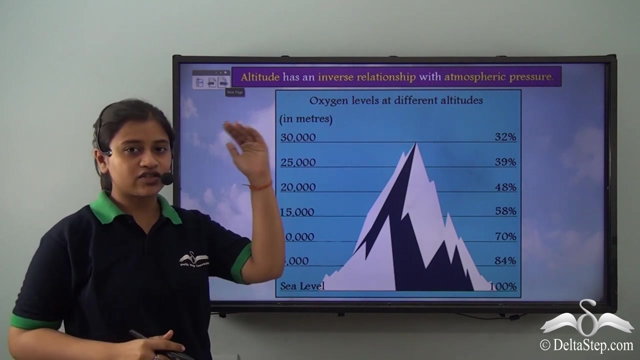 that the concentration of air molecules is more on the lower layers and is less on the upper layers, So the amount of oxygen is also less, and that is why, in order to travel such high altitudes, they carry oxygen cylinders. So we have been discussing since then that as we go up higher in the altitude, the atmospheric 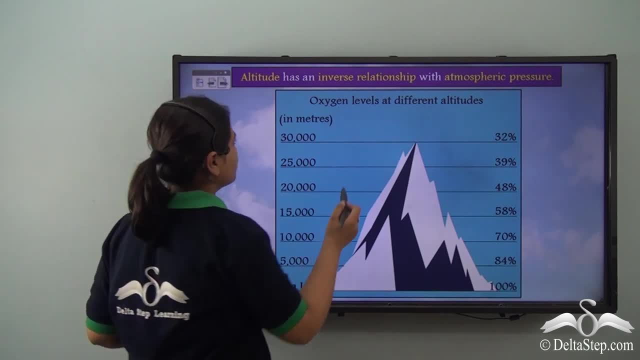 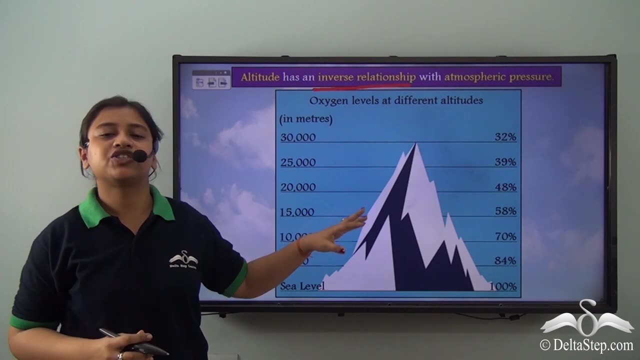 pressure decreases. So we can say that altitude has an inverse relationship with atmospheric pressure. So now that the atmospheric pressure is lower in the upper regions and higher in the lower regions, The concentration of air molecules down in the upper regions is less. So in this range atmospheric pressure is less Because atmospheric pressure is more. 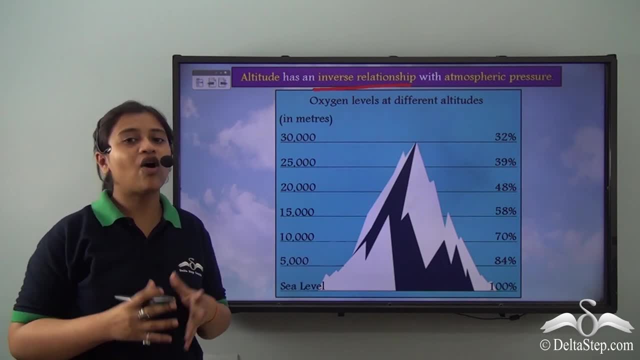 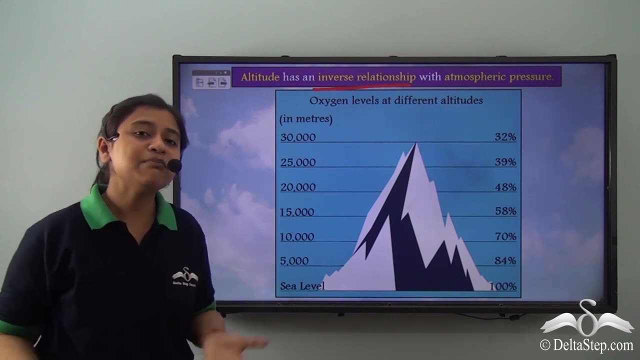 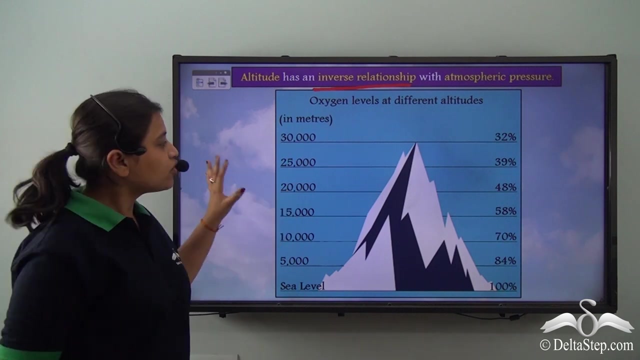 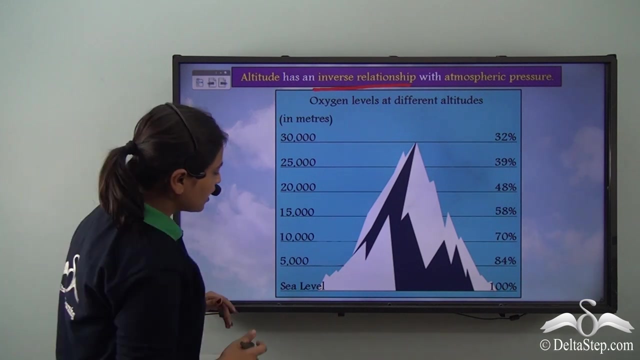 of air molecules is also lower or lesser in the high altitudes and more on the lower layers of the atmosphere. This only means that the oxygen level tends to decrease as we go higher up in the altitude. So looking at this particular image, it shows us the difference in oxygen level as we go higher up, So at sea. 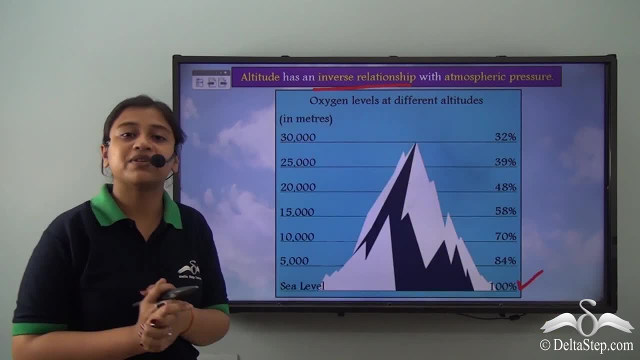 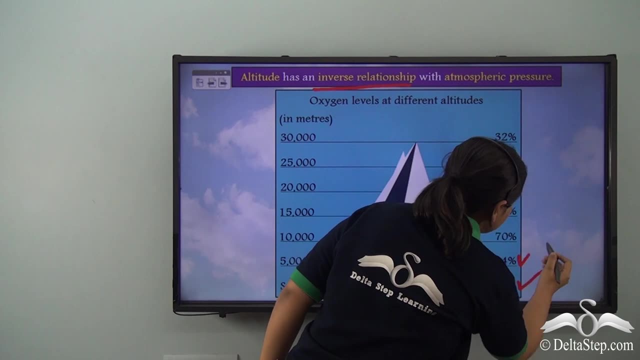 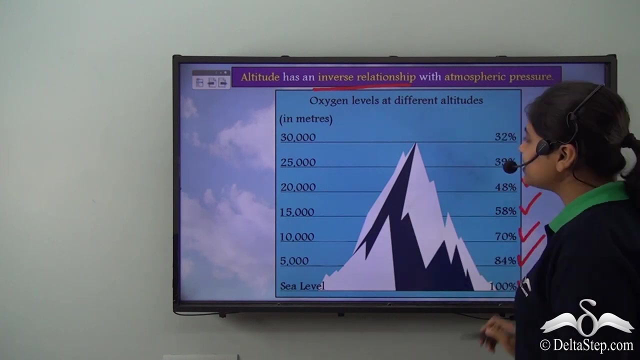 level, the oxygen is hundred percent. As we go up higher, 5000 meter above the sea level, the oxygen level is 84 percent. Then as we go up higher, at 10,000 meters, it is 70 percent, Then at 15,000 it is 58 percent, In 20,000 it is 48 percent. In 25,000 it is. 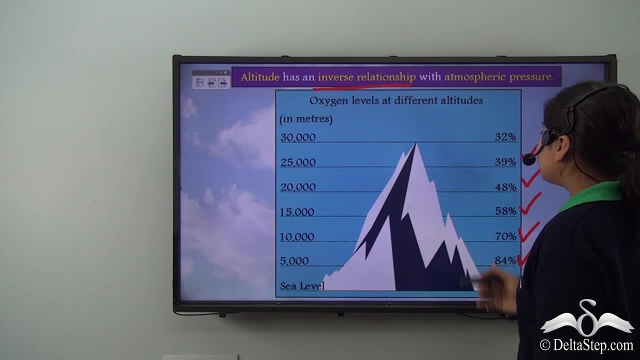 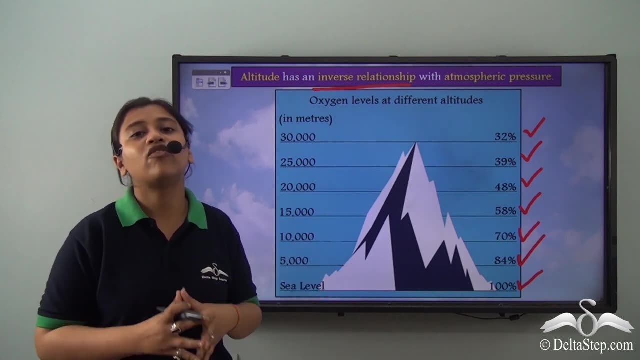 39 percent and in 30,000 it is 36 percent. So the temperature at 30,000 meters above sea level is 32 percent oxygen. So you see that there's a huge decrease in the level of oxygen at 30,000 meters above sea level, right? So here we understood that atmospheric. 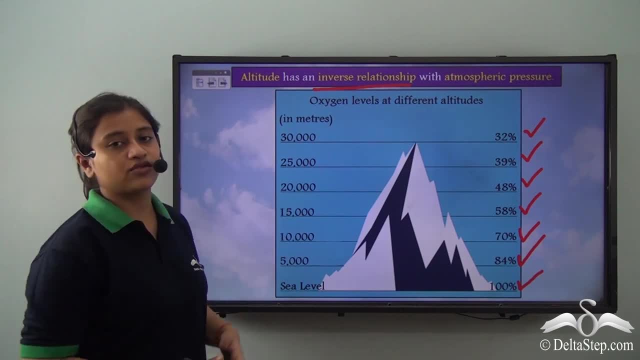 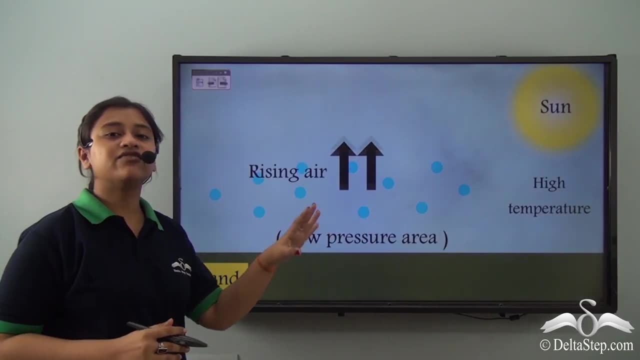 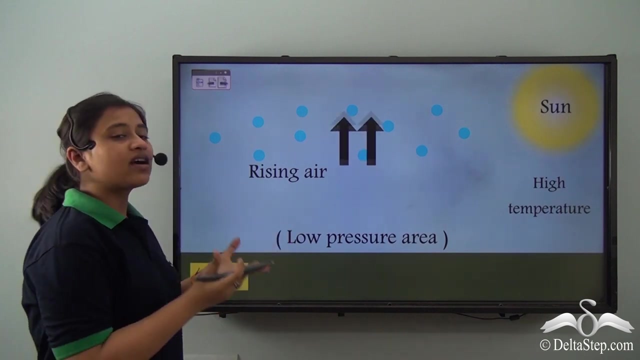 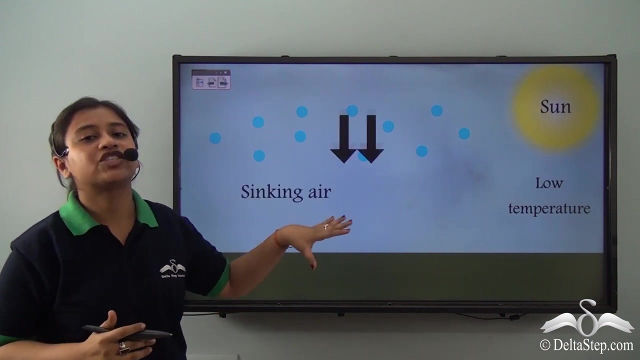 pressure has an inverse relationship with altitude. So now how does this work? So in land where temperatures are very high, the molecules tend to move away from each other, the space between them increases and they become light or less dense and rise above right, so it becomes a low-pressure area. but in regions where 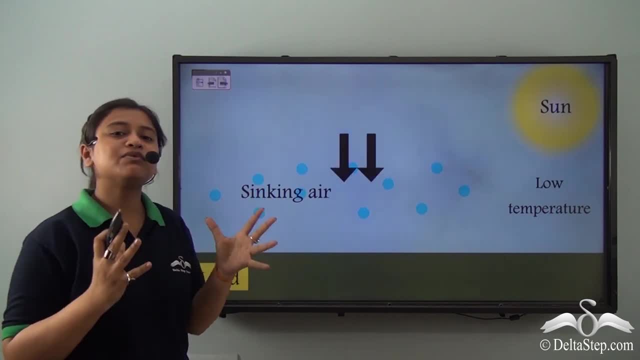 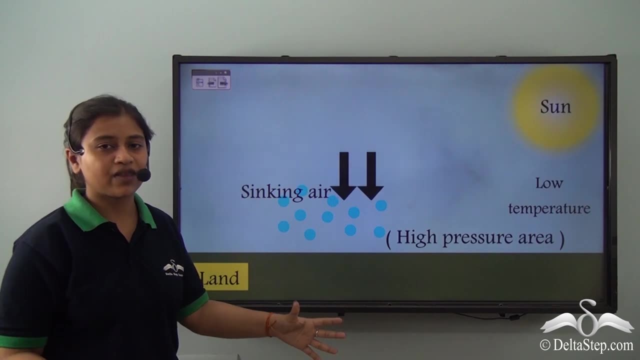 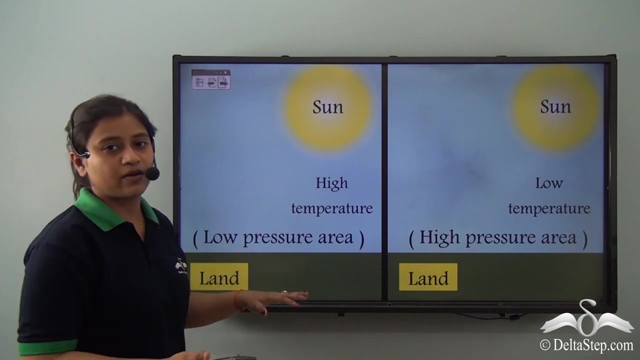 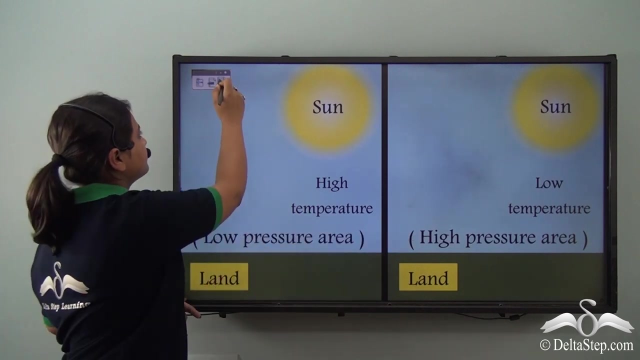 temperatures are very low. there, the spaces between the molecules decrease and they become more dense and they sink down, creating a high-pressure area. right? so this is how this works. so this is how temperature is related to atmospheric pressure. higher temperatures means low-pressure area. lower temperatures means high-pressure area. so now that we have 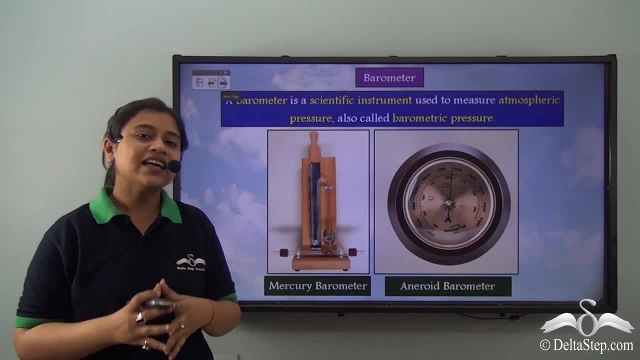 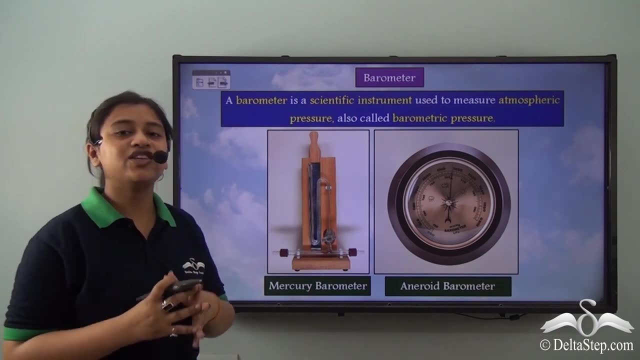 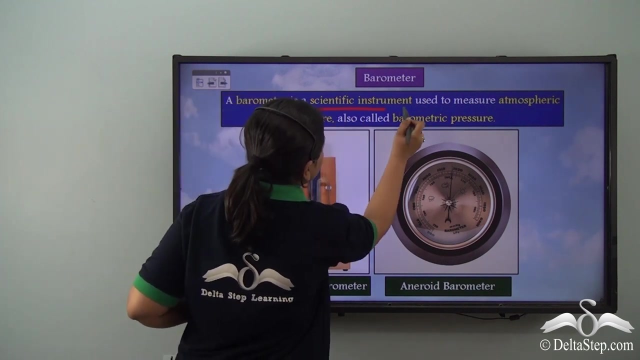 understood what atmospheric pressure is. let's see what is used to measure this atmospheric pressure. well, a barometer is used to measure the atmospheric pressure of place. so breathing is a scientific instrument used to measure the atmospheric pressure pressure, and it is also called the barometric pressure. 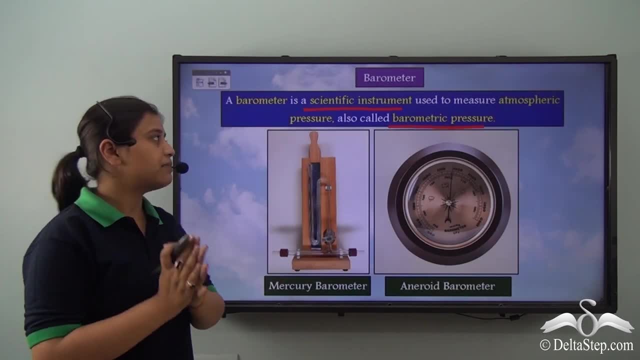 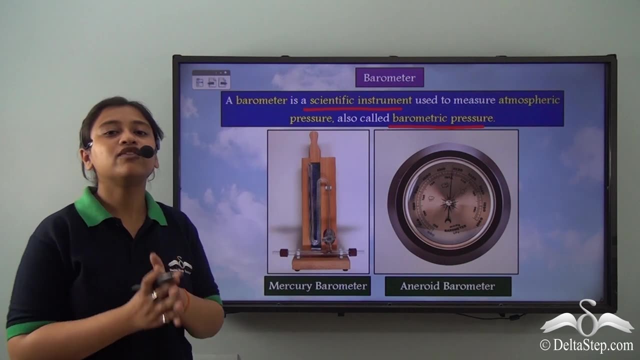 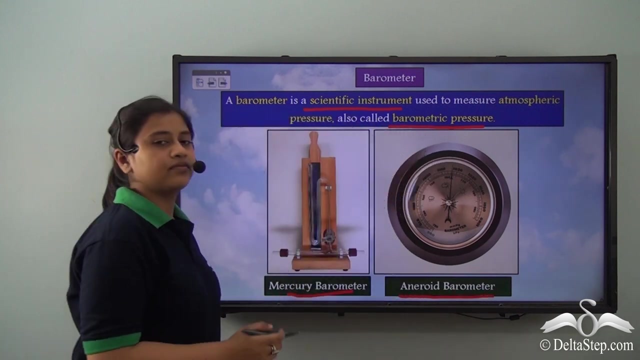 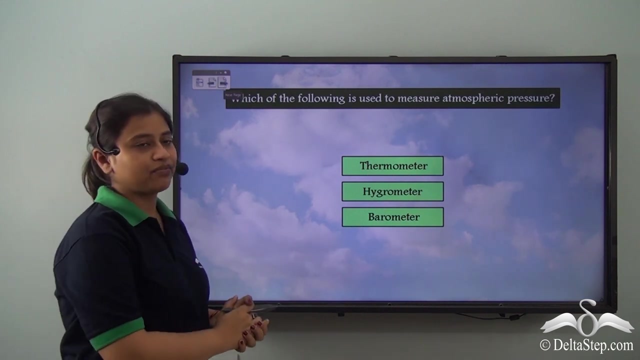 So atmospheric pressure, or barometric pressure, is measured with the help of a barometer, which is a scientific instrument. Now, this barometer could be of two types: mercury barometer and aneroid barometer. So before moving on, could you help me answer this question? 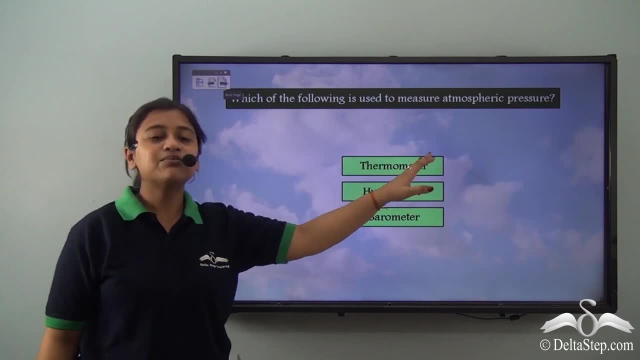 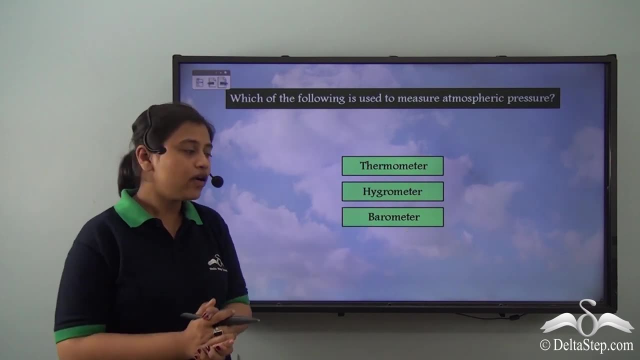 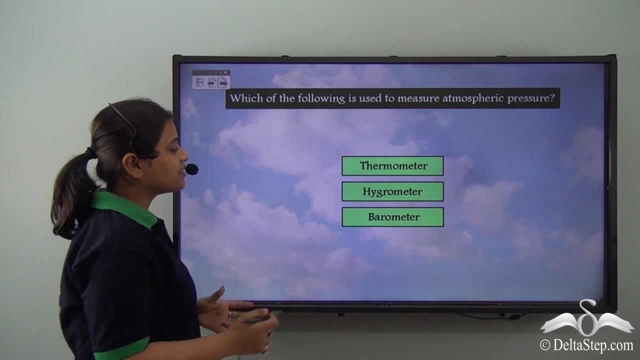 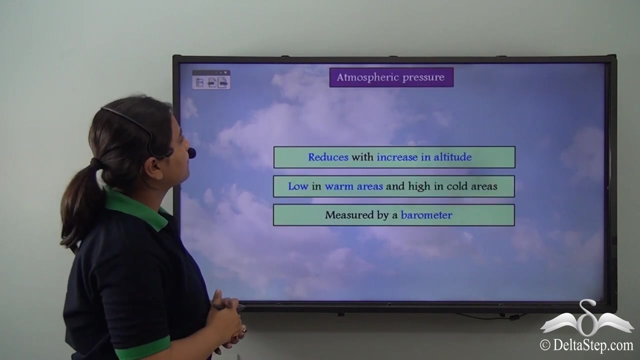 Which of the following is used to measure atmospheric pressure: Is it a thermometer or is it a hygrometer or is it a barometer? Yes, we just learned that it is a barometer that is used to measure the atmospheric pressure. Now, so far we understood what is atmospheric pressure. 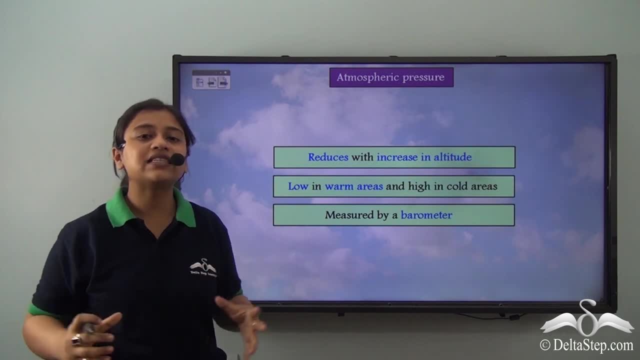 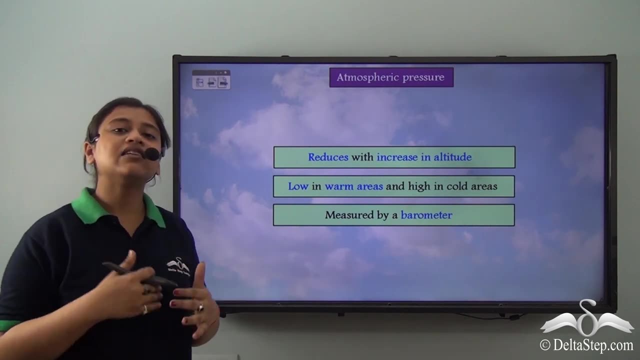 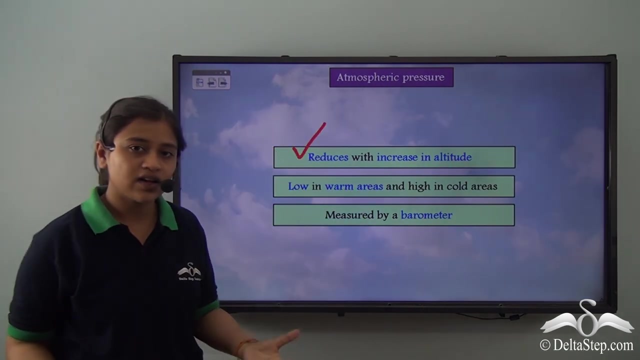 It is the weight of the air on a unit area of the earth's surface right, and we understood that atmospheric pressure has an inverse relationship with altitude, So it reduces with the increase in altitude and vice versa. We also understood that atmospheric pressure is low in warm areas. 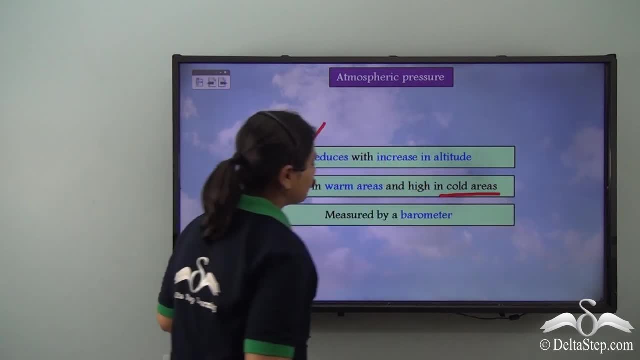 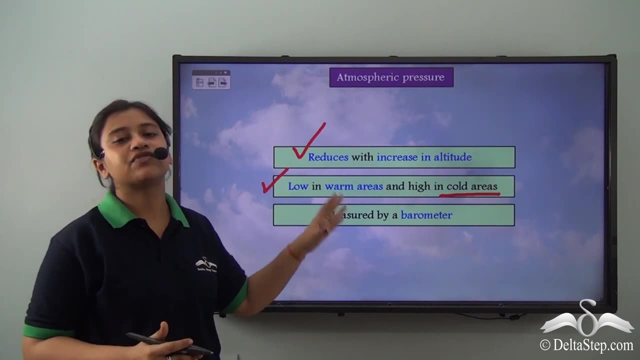 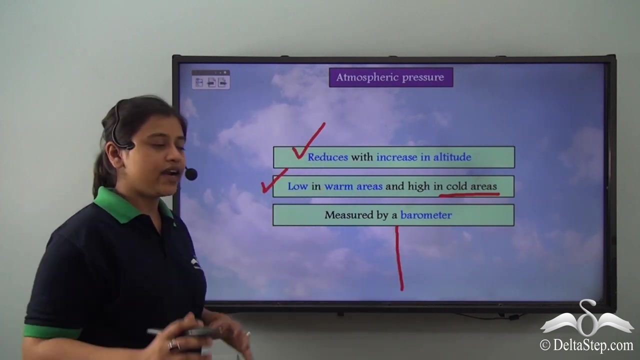 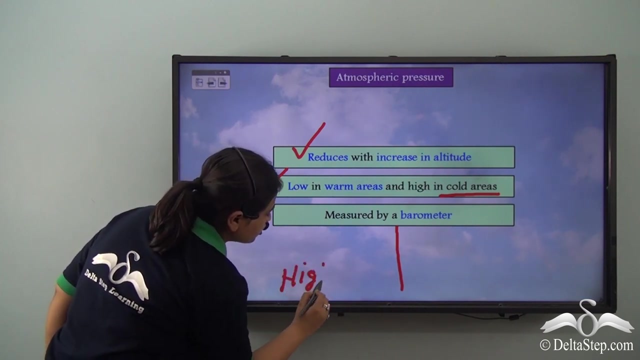 and it is high in cold areas. We further understood that it is a barometer, that is, a scientific instrument that is used to measure the atmospheric pressure. So suppose if we divide this small region into two halves, where this is a area with high pressure? So the temperature here? 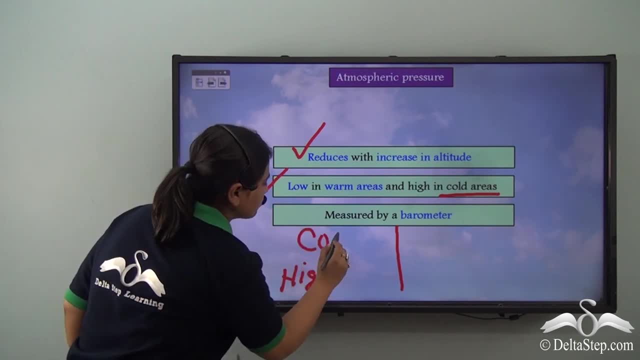 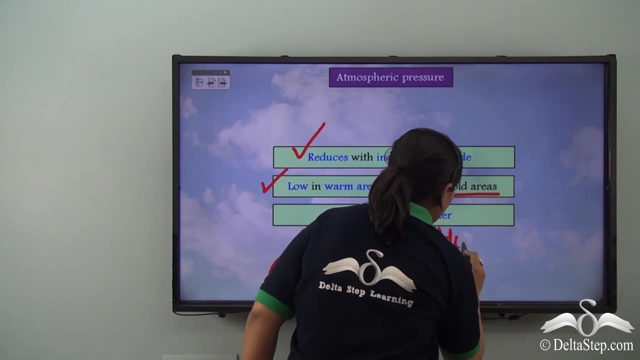 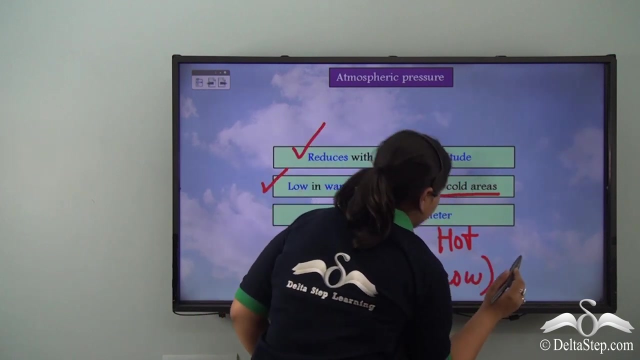 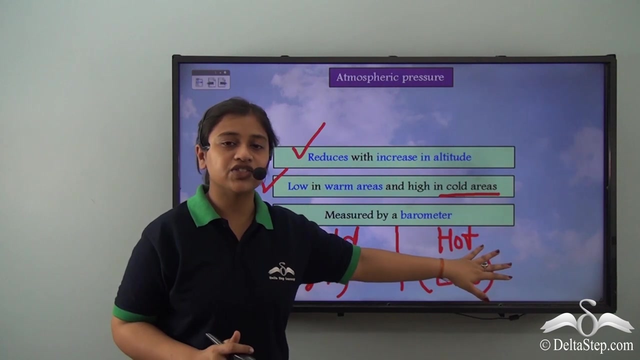 is very low, So it's a cold region, while this is a hot region, where the temperature is very high but the pressure is very low. Okay, so this is a cold region with low temperature and high pressure, and this is a hot region with high. 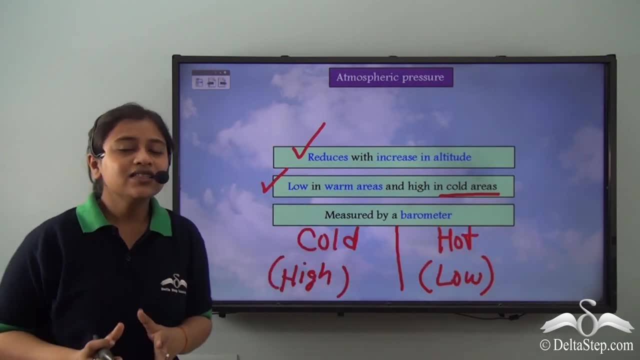 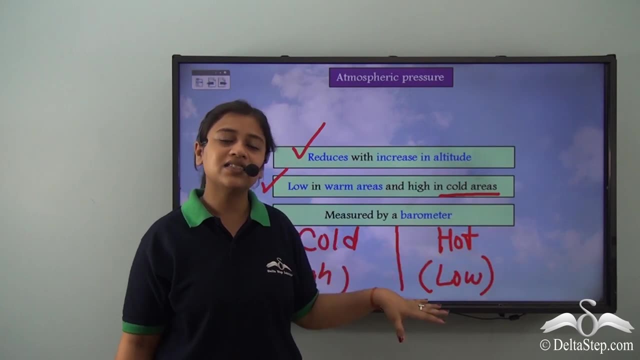 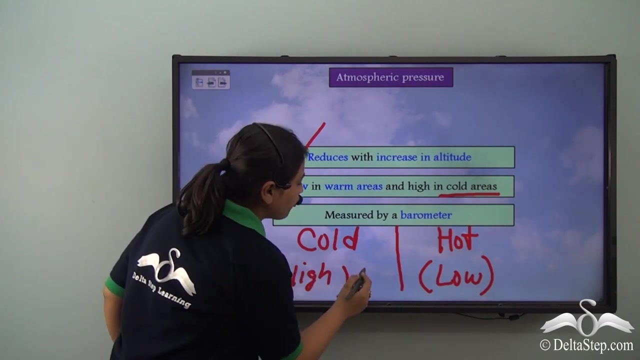 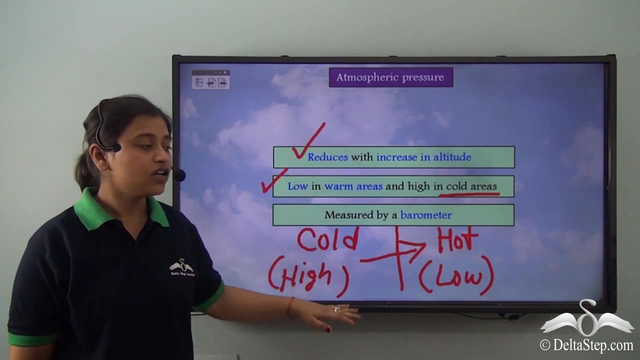 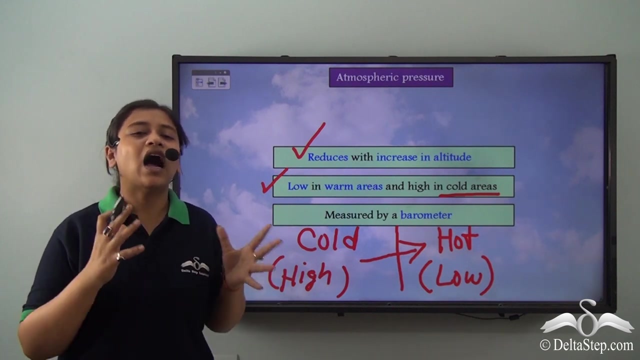 temperature and low pressure. So it is a tendency of the wind that is moving air to get attracted to low pressure areas or areas that are of high temperature. So what generally happens is winds move from colder regions to hotter regions or from high-pressure area to low pressure area. right, So this is very simple, but how does? 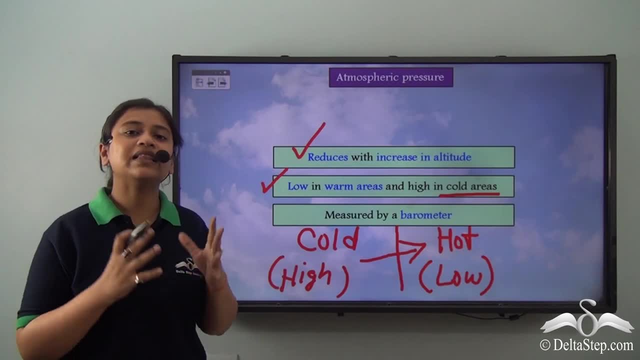 it affect or how does it influence weather? Well, when these winds move over water bodies that are regions with low temperature, they tend to carry moisture water bodies that are regions with low temperature, they tend to carry moisture water bodies that are regions with low temperature. they tend to carry moisture with them. So these moisture laden winds move from this high-pressure area to the low-pressure area where they condense and, on meeting an obstruction, they precipitate. So we can simply say that winds bring rainfall when they move from high-pressure area to low-pressure area, and these are not any winds, but winds that carry moisture. So let's see how does this work. 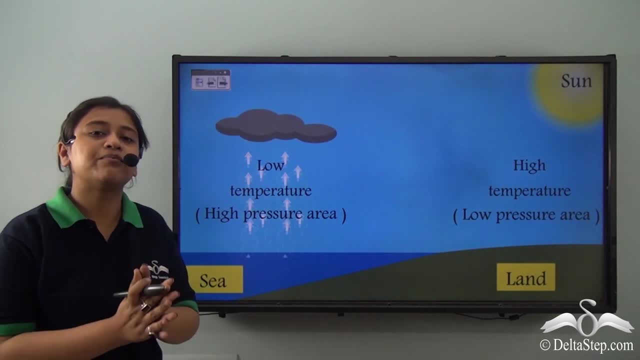 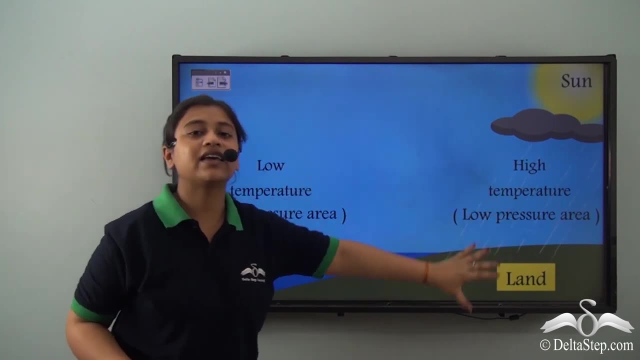 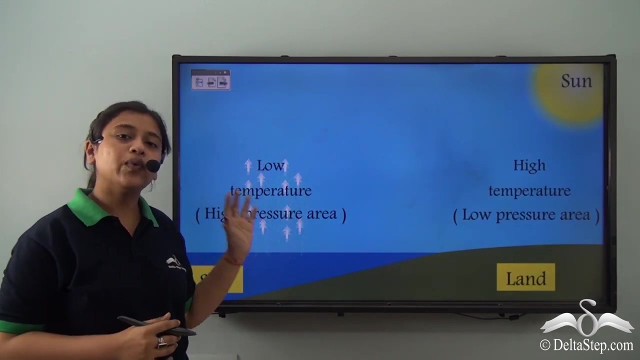 So is an area C, where the temperature is very lower-so it's a high-pressure areaSo the wind from here moves to the low-pressure area, carrying moisture, and then it condenses and on meeting an obstruction, they precipitate. So this is how wind affects, or influences, weather. So what do? 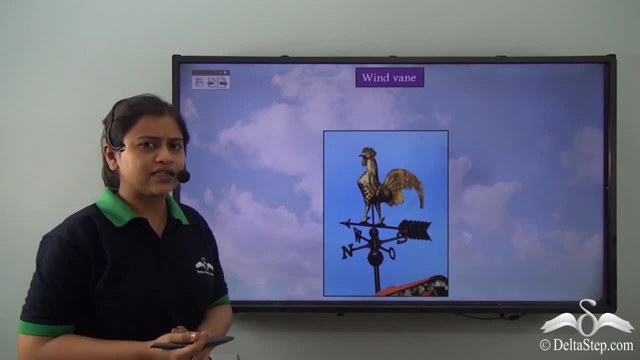 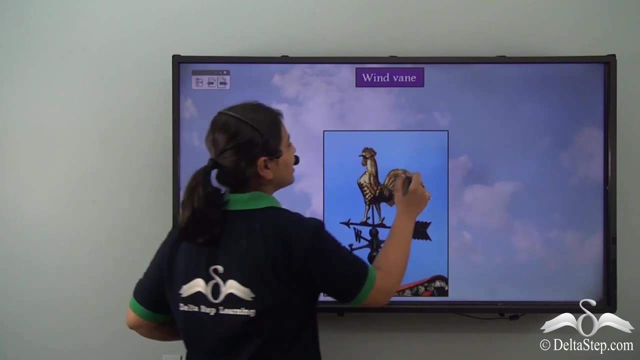 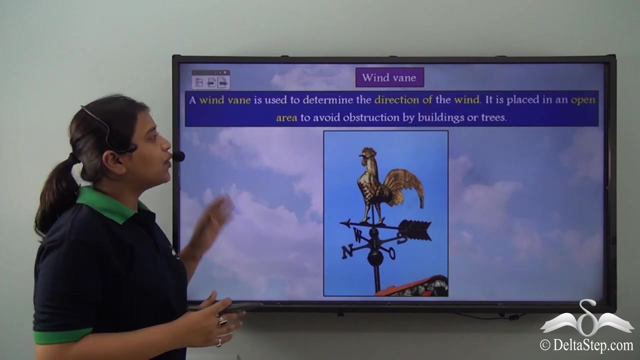 you see here, You see a chicken, but is it eatable? No, No, this is a instrument, a wind instrument, and this is known as a wind vane. So how is it used? Well, a wind vane is used to determine the direction of the wind. It is placed in. 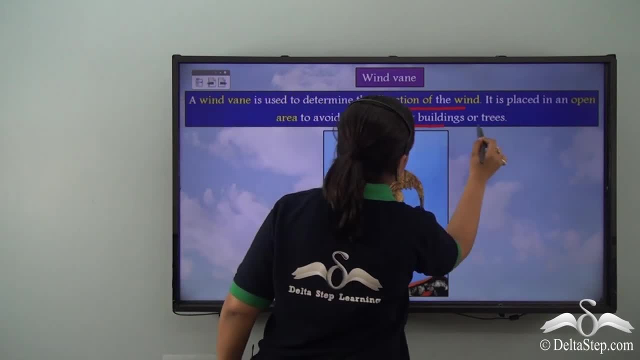 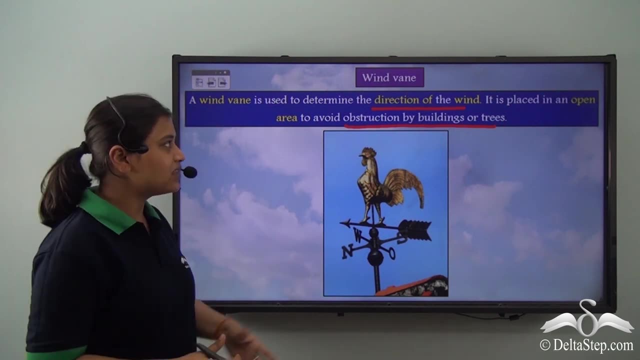 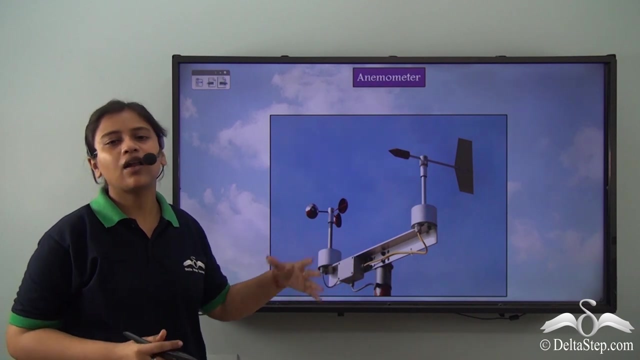 an open area to avoid obstruction by buildings or trees. So a wind vane is a wind instrument that is used to determine the direction of the wind. Well, this is another wind instrument. Now, what does this do? We have wind vane to determine the direction of the wind, but what? 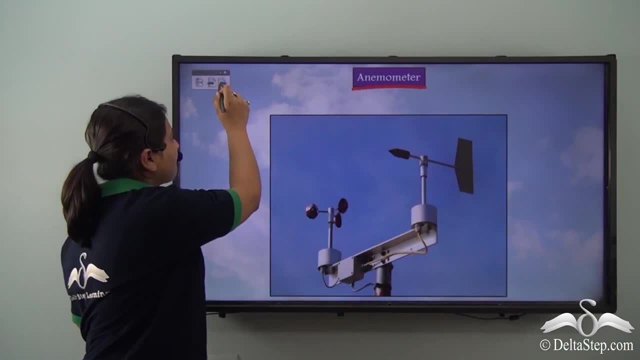 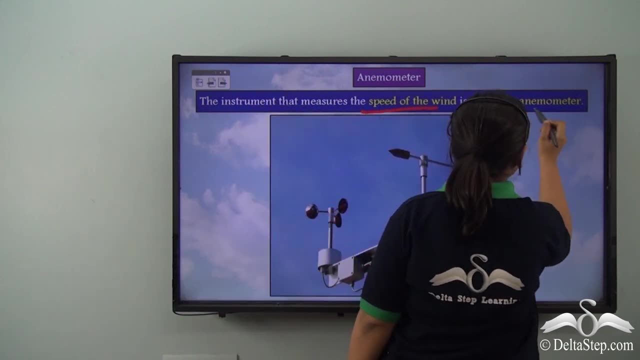 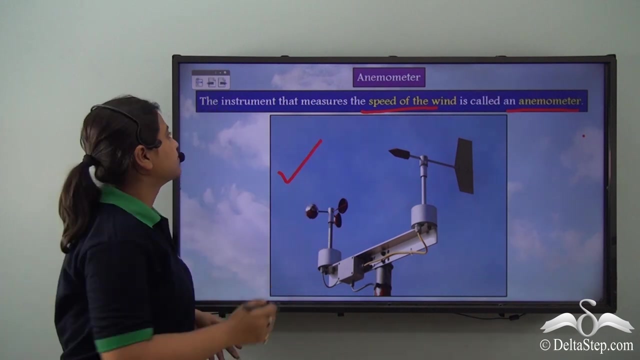 is an anemometer. Well, the instrument that measures the speed of the wind is called an anemometer. So this is an anemometer which measures the speed of the wind. speed of the wind. So far we have learnt about all these different weather. 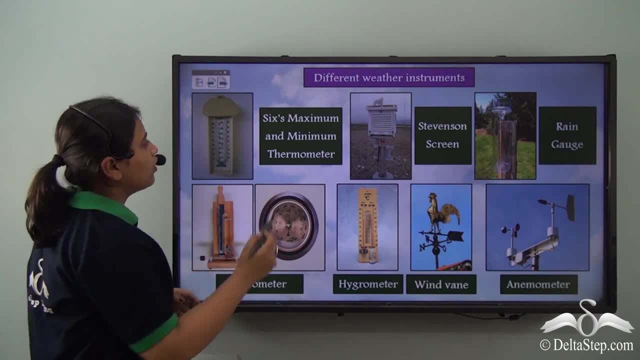 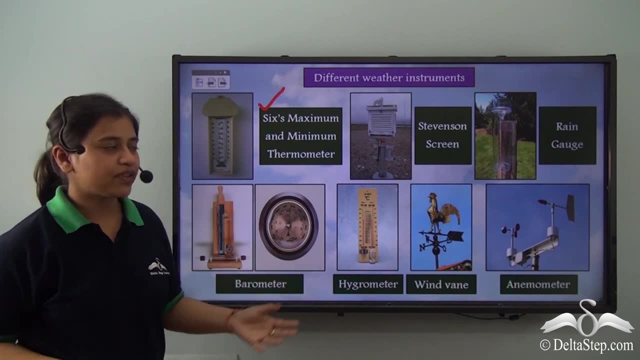 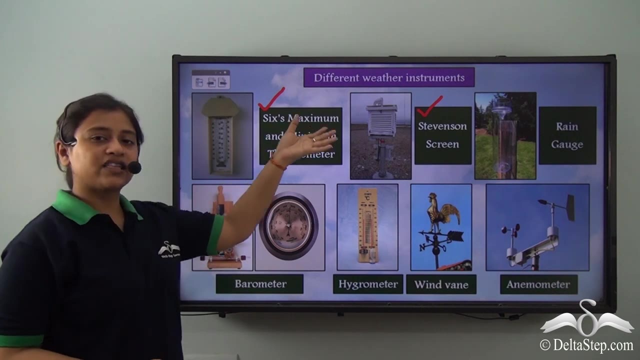 instruments. Let's take a recap. We learnt about sixes maximum and minimum thermometer that helps us record the temperature of the atmosphere. We also learnt about Stevenson screen that protects or provides a shade to the sixes maximum and minimum thermometer. Then we learnt about the rain gauge that helps. 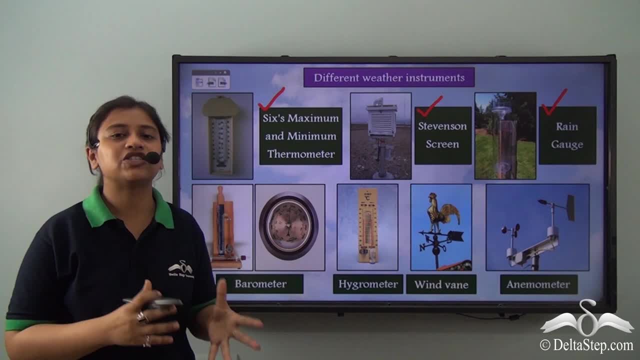 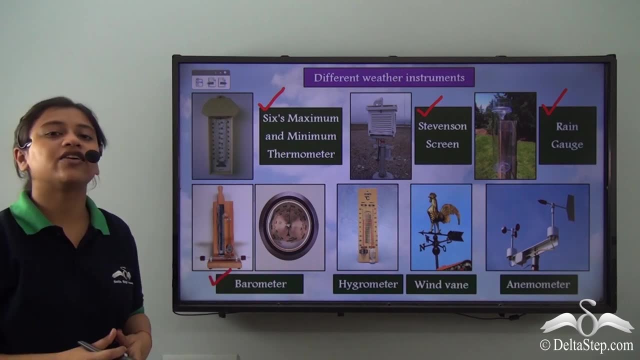 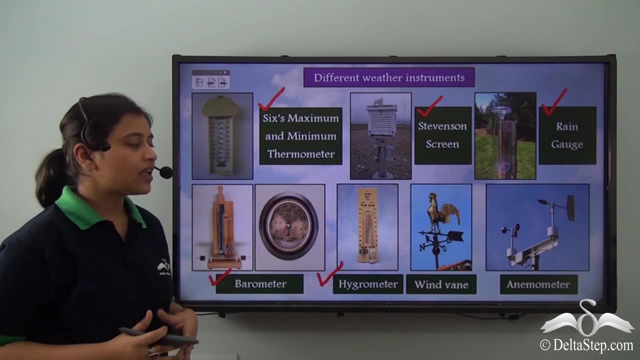 us measure or record the amount of rainfall in a particular area at a particular time. We further learnt about barometer that helps us record atmospheric pressure. Then we learnt about hygrometer that measures humidity. Then we learnt about wind vane and anemometer, where wind vane helps us. 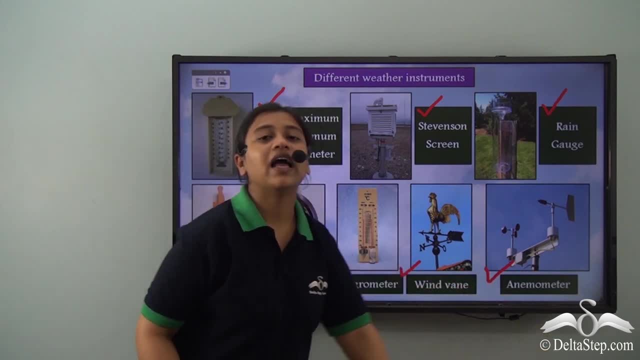 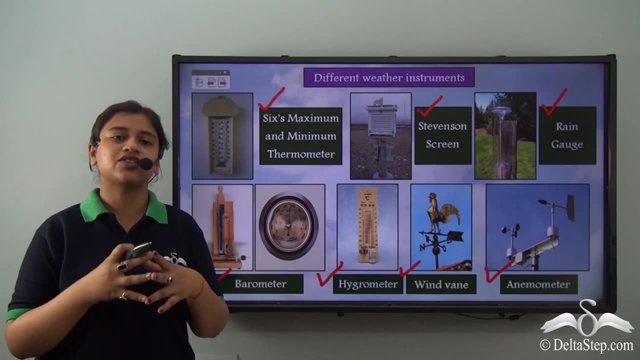 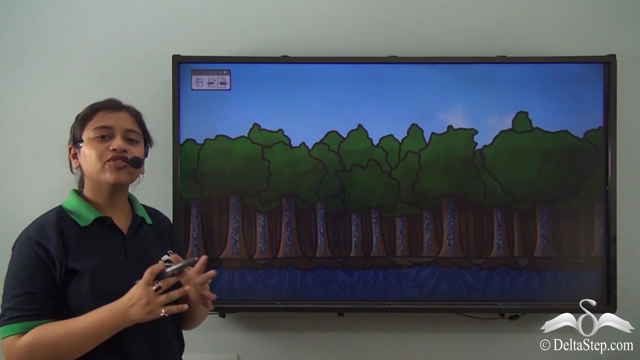 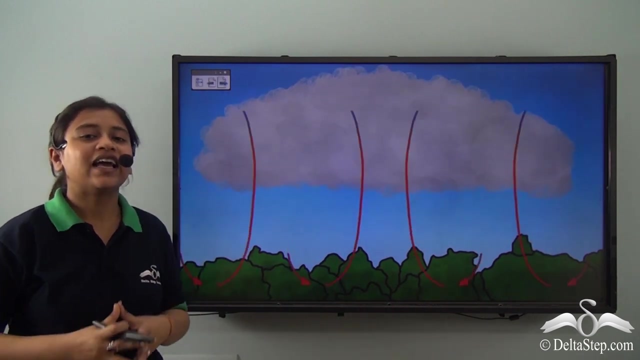 understand the temperature, the direction of the wind, and anemometer helps us understand the speed of the wind. So these are the different weather instruments that helps us record and study different weather conditions. Have you ever heard of an amazing weather phenomena known as the 4 o'clock showers? Well, yes, in regions that are located on or near the equator, they have an equatorial type of climate. So those regions that are forested on the equatorial region tend to evaporate huge amount of water or moisture from the trees into the atmosphere. So because they receive direct rays of the sun, So on. 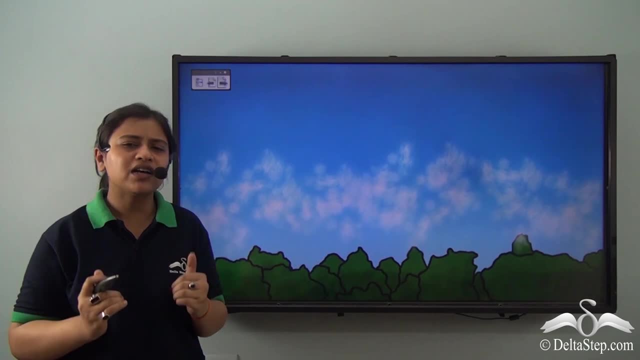 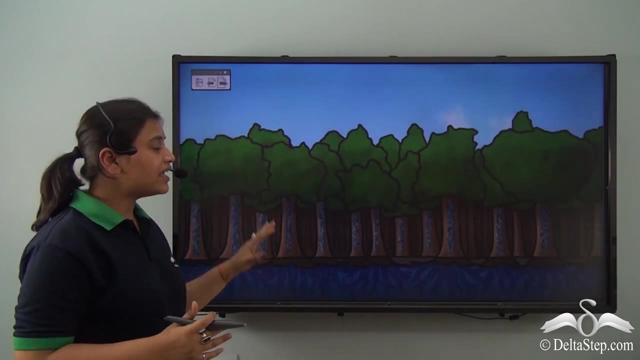 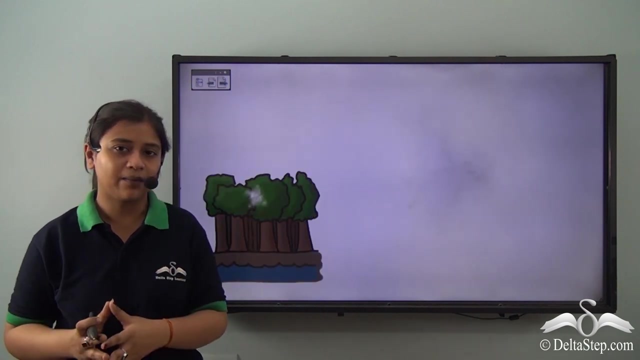 receiving direct rays of the sun, the evaporation rate is much faster and at a very large amount. This evaporation of sun leads to cloud formation, and these forested areas in the equatorial region tends to receive rainfall at around four o'clock every day, And this is known as the 4 o'clock. 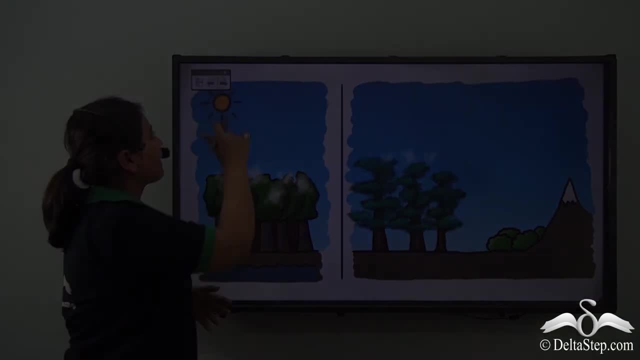 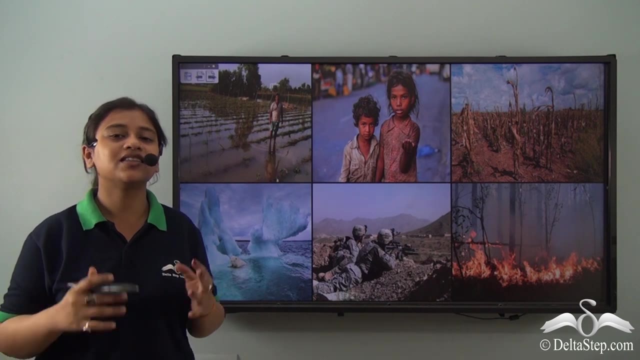 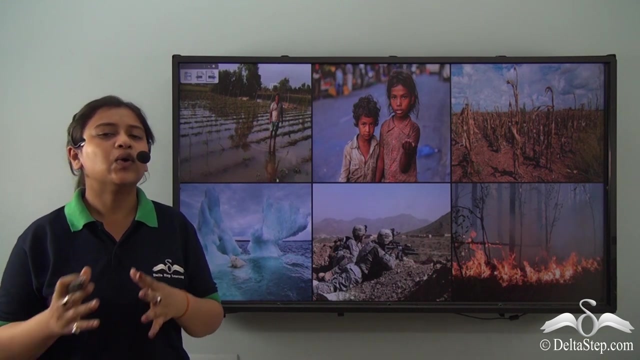 shower, Isn't that amazing. So we just learnt about that amazing weather phenomena that is, the 4 o'clock showers that occurs in the equatorial region. but what if there were no trees at all? What if we cut down all the trees? Will? 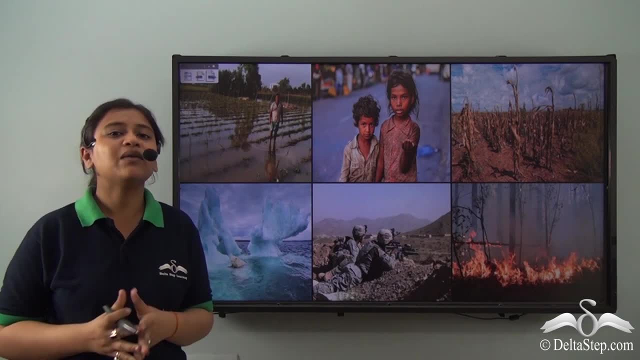 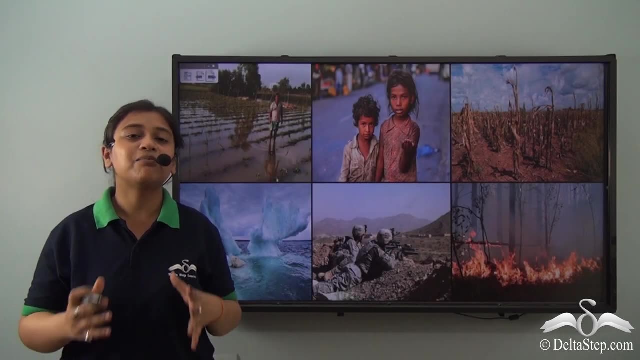 will this four o'clock shower still happen? No, There will be nothing left. There will be no phenomena, no amazing phenomena that we could admire. So it is very sad that planting a tree has almost become mandatory. Deforestation has happened to such an extent that it has. 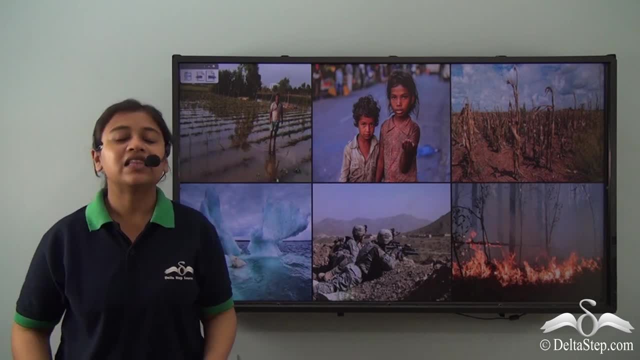 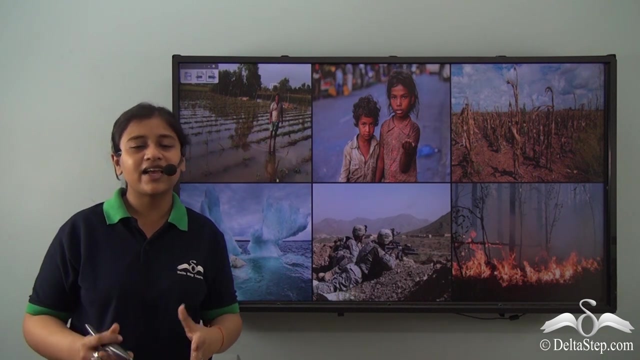 affected the climate of the earth as a whole. The temperature of the earth has increased, leading to global warming, and many other human activities, like the working of industries, the agricultural activities where we use chemical fertilizers and pesticides. all of this has led to increase in the greenhouse emission also. 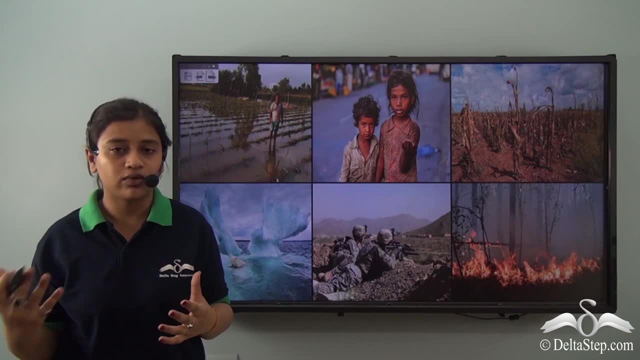 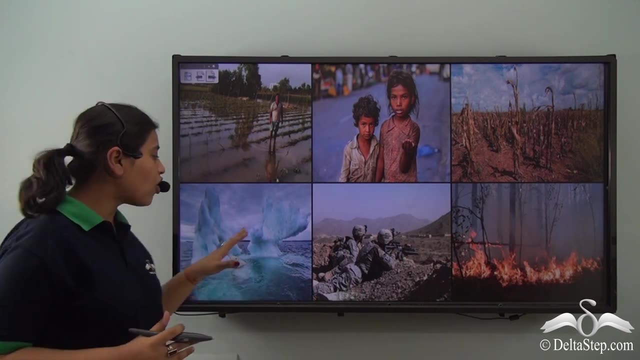 So we see that we have led to the increase in global warming. Global warming, in turn, has had negative impact on the earth. It has led to the loss of habitat in polar regions where ice beds are not available. So we have seen that there has been an increase in global warming. Global warming, in turn, has had negative impact on the earth. It has led to the loss of habitat in polar regions where ice beds are not available. So we have seen that there have been an increase in global warming. Global warming, in turn, has led to the loss of habitat. 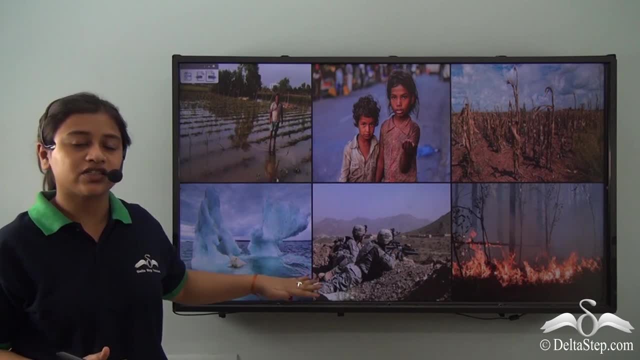 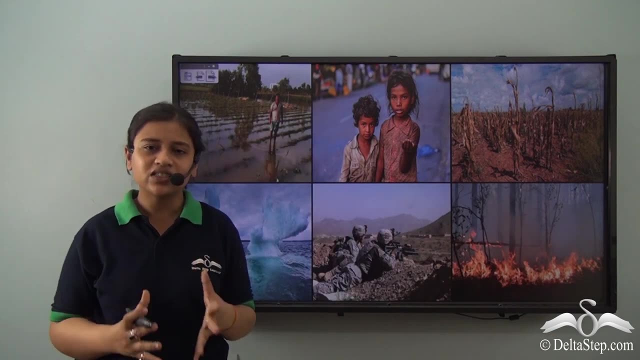 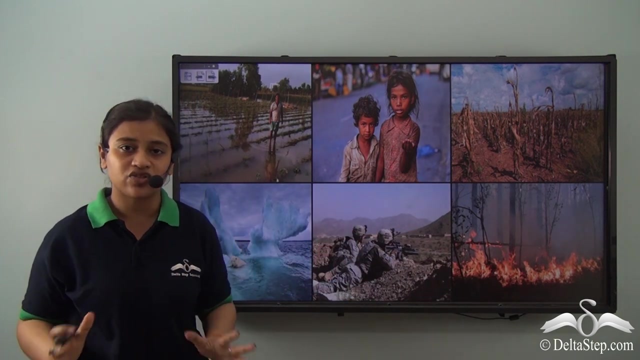 in polar regions where ice beds are not available. So we have seen that there has been an increase in global warming, in particular fern and skank animals, but they do not pose any major problems. So we have seen that the Darwin law has also said that this global warming can be calendarized for over a decade. So 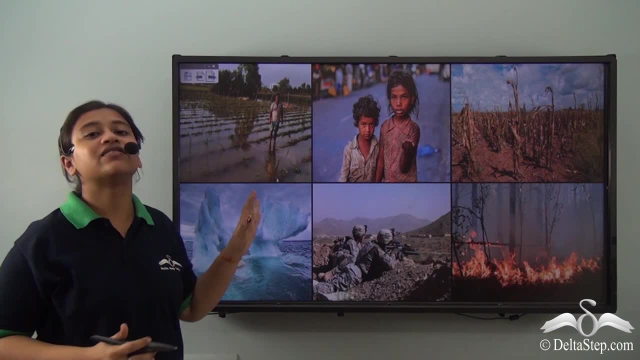 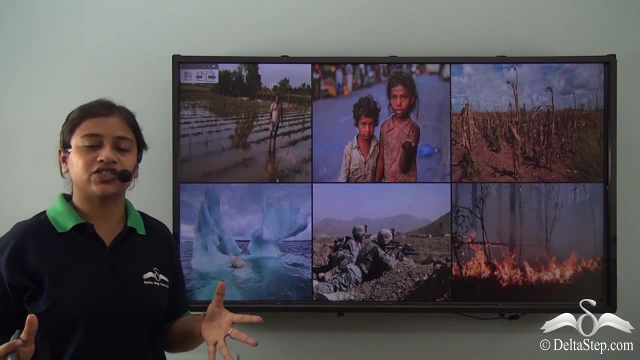 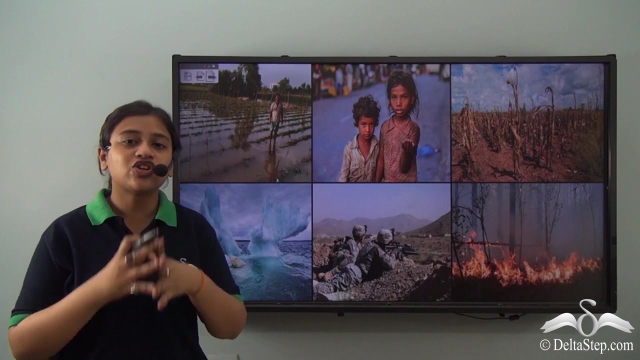 the global warming check has again been an eight month checklist for them, Butก, as you watch it on YouTube, it is usually again given two minutes, three minutes of when suffering from drought, the crop cultivation is being negatively affected. the production of crops is not as expected, so there is shortage of food. 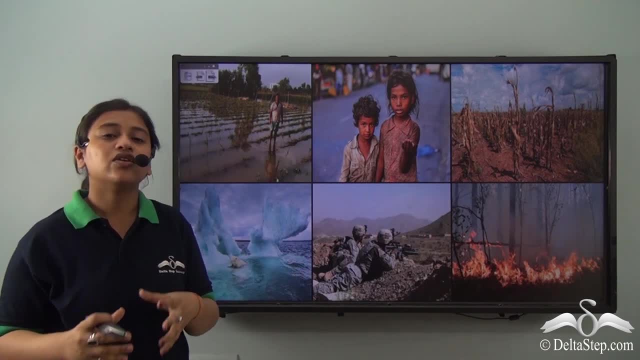 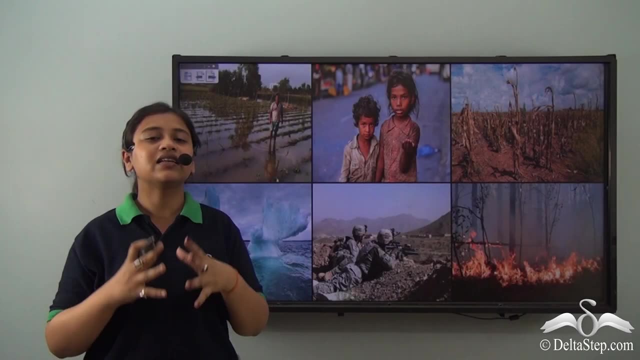 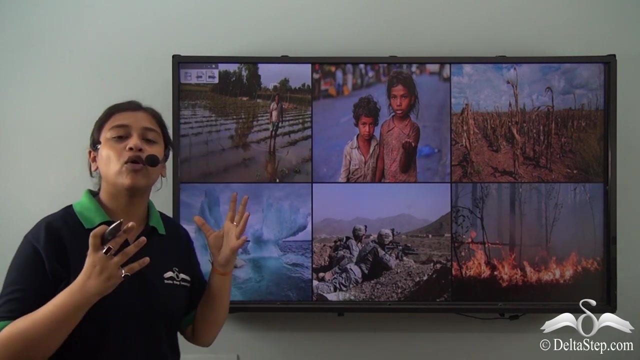 many other such things, is leading to limiting of resources, which may lead to poverty and wars between nations. so you see that climate that affects the lifestyle of people across the world may also affect our lives, both positively and negatively, and it is on us that we be responsible enough and not over. 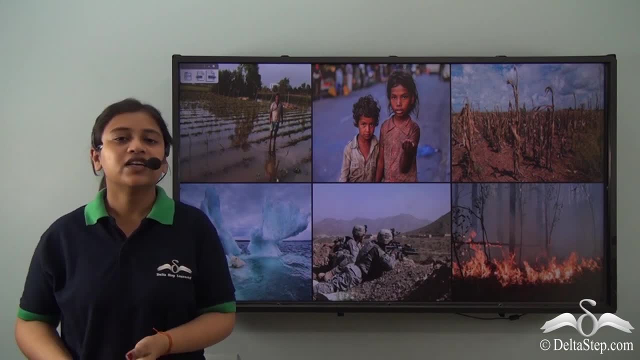 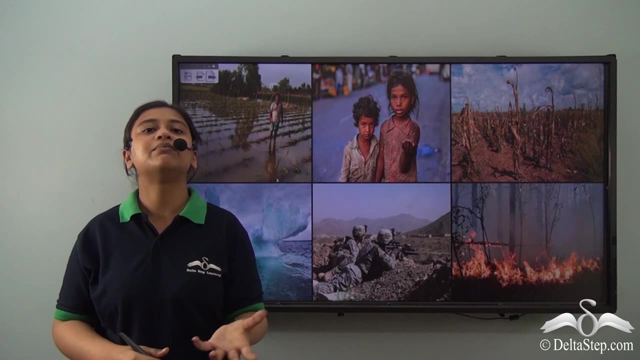 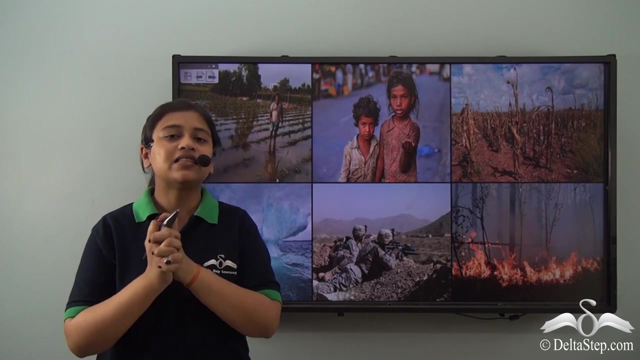 exploit the resources that are already so limited. so you see that today in this video we have learned about atmospheric pressure as an important element of weather and also wind as an important element that influences weather. we summarized or recapped all the weather instruments and then we also learned.